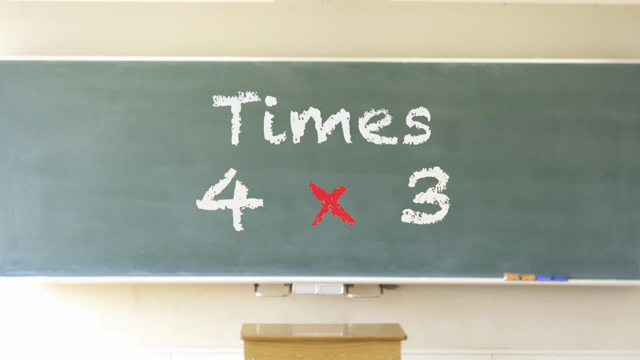 Here is how you will read it: 4 times 3.. Factors: The numbers that you multiply together are called factors In the problem. 2 times 5, the factors are 2 and 5.. Product: The product is an answer for a. 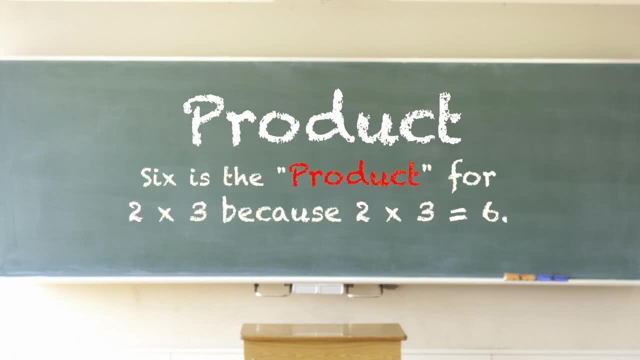 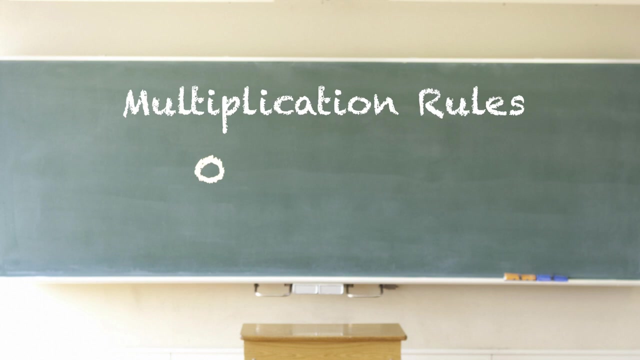 multiplication problem: 6 is the product for 2 times 3, because 2 times 3 equals 6.. Here are some multiplication rules. Any number is multiplied by zero is equal to zero. So zero times five equals zero. Any number that 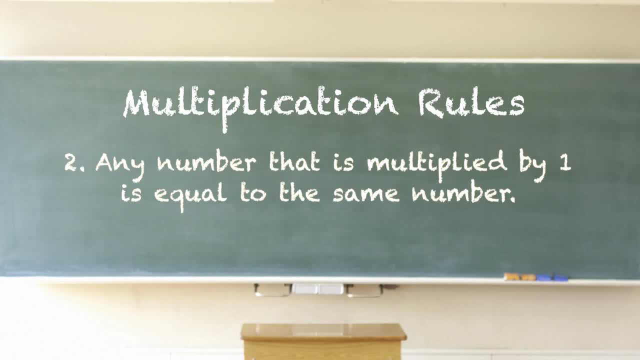 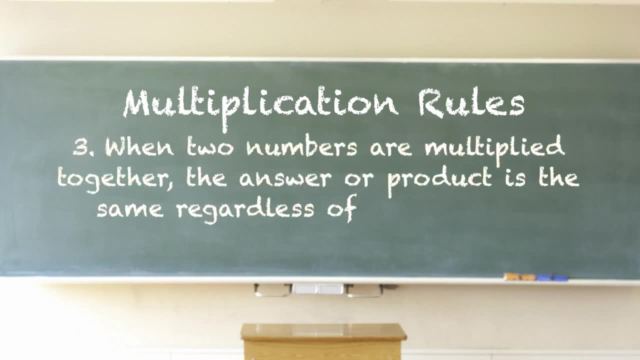 is multiplied by one is equal to the same number. For example, one times three equals three. When two numbers are multiplied together, the answer or product is the same, regardless of the order of the factors. For example, two times three equals three times two, Both. 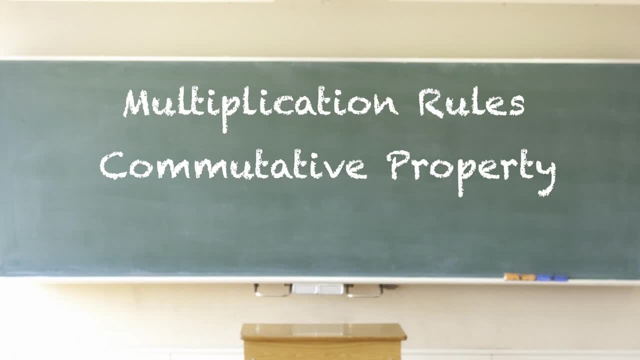 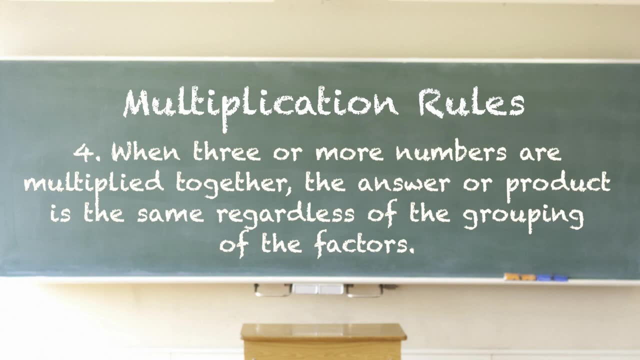 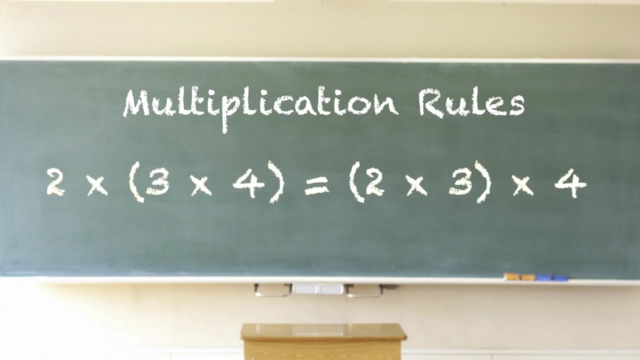 are equal to six. This is called the commutative property. When three or more numbers are multiplied together, the answer or product is the same, regardless of the grouping of the factors. Two times the grouping of three times four is equal to the grouping of 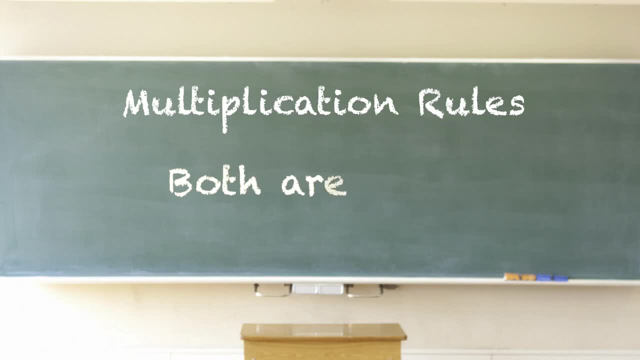 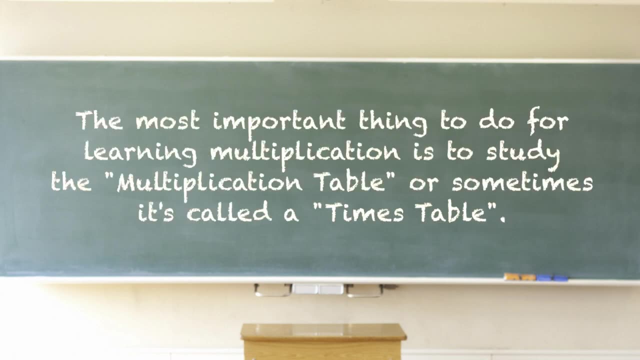 one 2 times 3 times 4.. Both are equal to 24.. This is called the associative property. The most important thing to do for learning multiplication is to study the multiplication table, or sometimes it is called a times table. The following shows you a multiplication table. 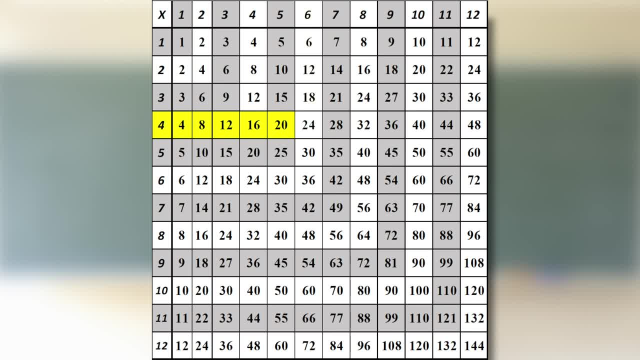 and how to use it. Notice where the 4 in the left column meets the 6 in the top column. This tells you that 4 times 6 is equal to 24.. Here are more examples: 1 times 3 equals 3.. 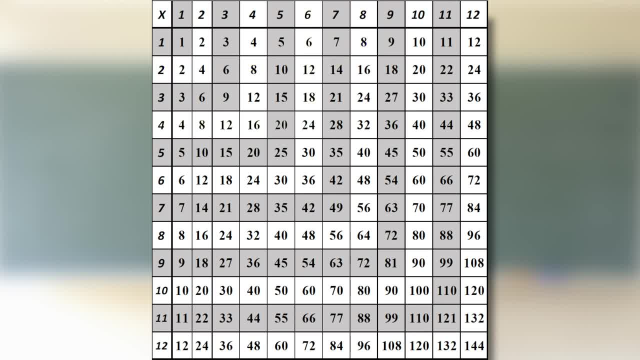 The product of 2 times 8 is 16.. The product of 3 times 5 is 15.. The product of 5 times 2 is 10.. What is the product of 12 times 10?? If you said 120, you're right, Remember.